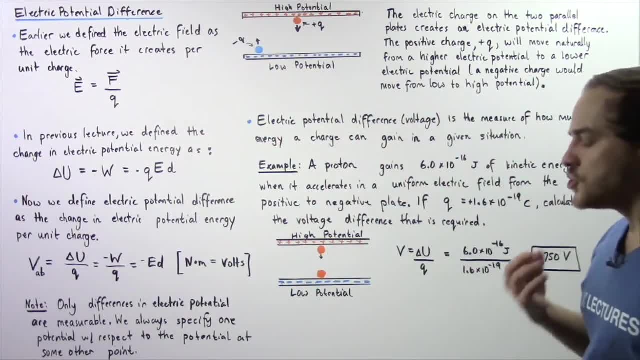 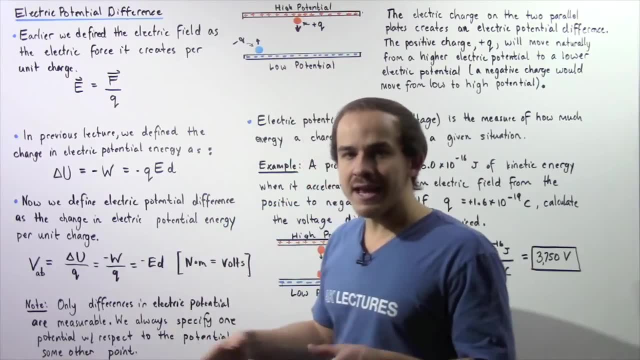 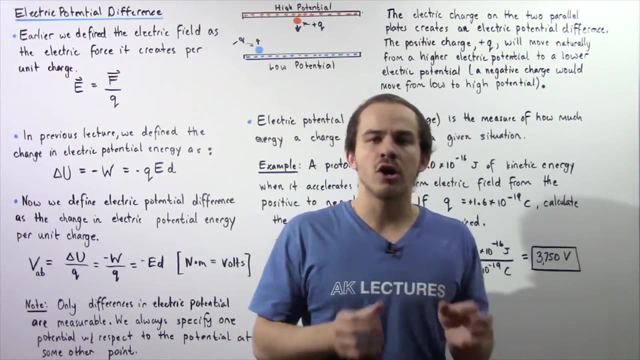 So in the previous lecture we defined the change in electric potential energy given by changing you between some point A and some point B as the negative quantity of work that is done by an electric force to move an electric charge over that distance from point A to point B. 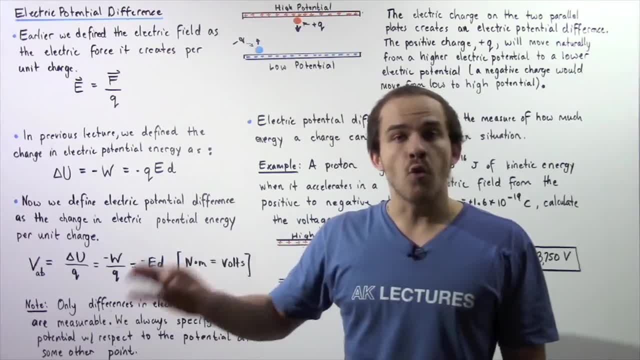 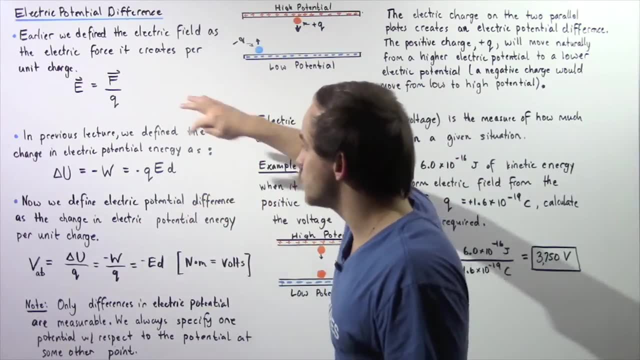 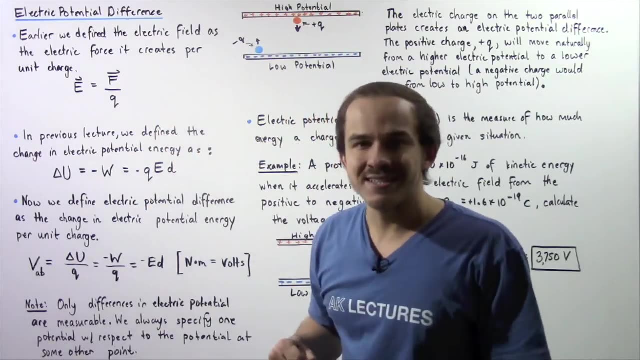 Now we also said: because our work is equal to force multiplied by distance and because the force is an electric force, that means the work is equal to Q, the charge multiplied by E, which is our force multiplied by our distance. So Q multiplied by E is the electric force. 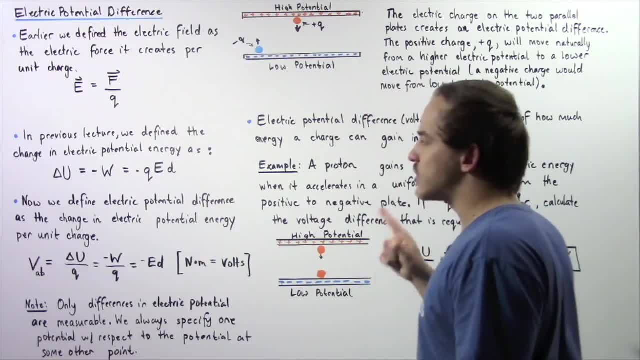 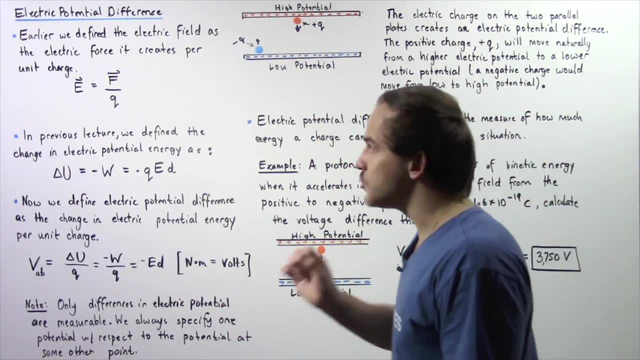 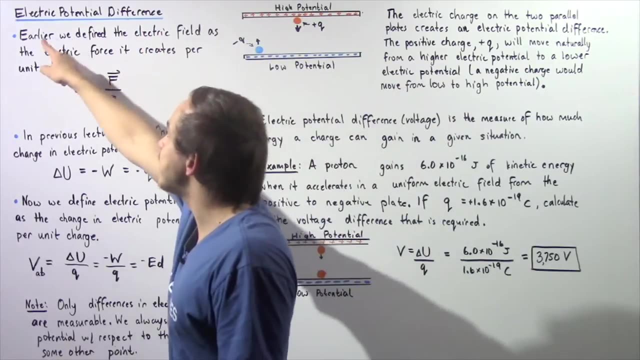 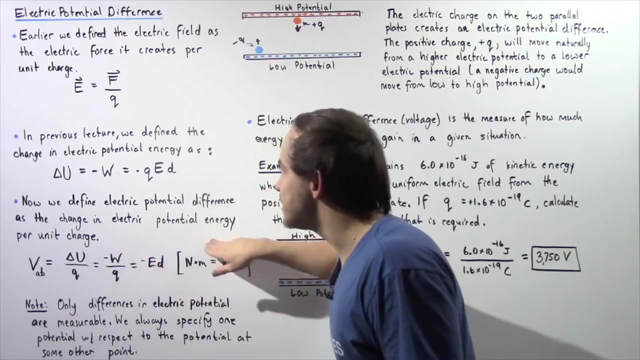 And this equation only works as long as our electric field is assumed to be constant. Now, in the same way that we found it useful to define the electric field as the force per unit charge, we defined something called the electric potential difference, or simply the voltage difference, as the change in electric potential energy given by changing you per unit charge. 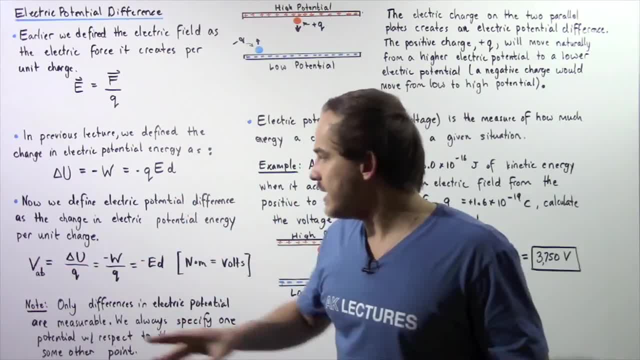 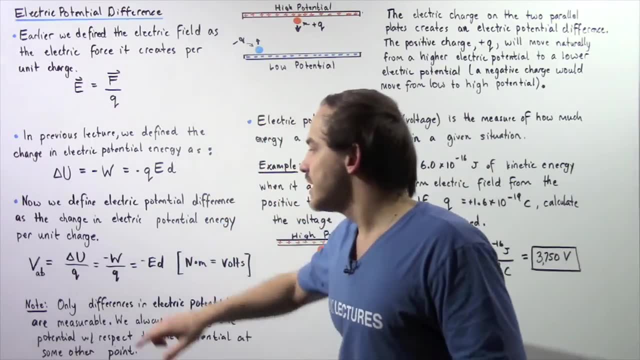 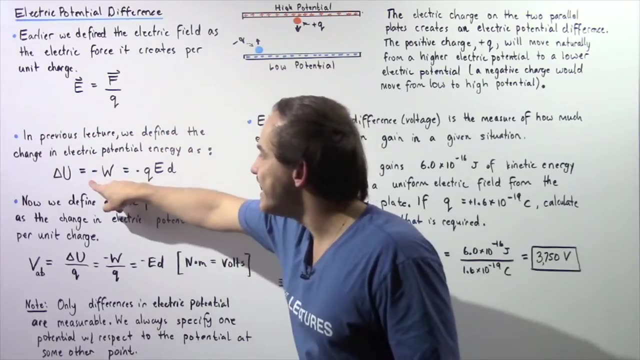 So the voltage difference between two points, A and B, is equal to the change in electric potential energy between those two points divided by the unit charge given by Q. Now we can replace our change in U with negative W, and we can replace negative W with QED. 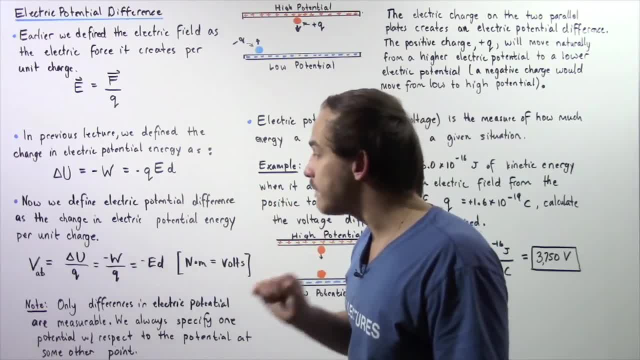 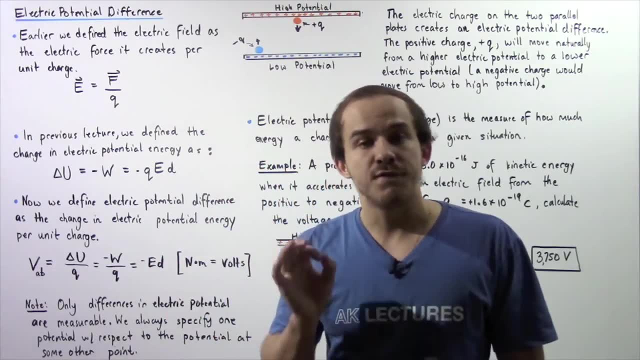 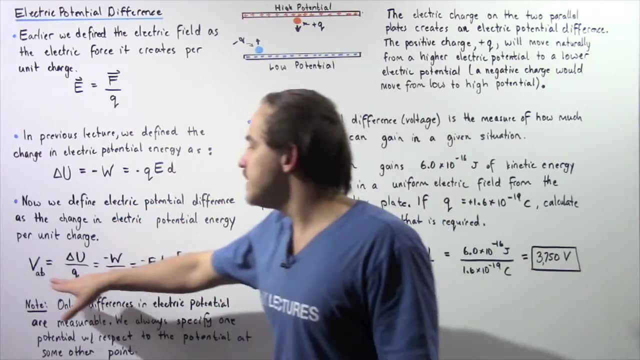 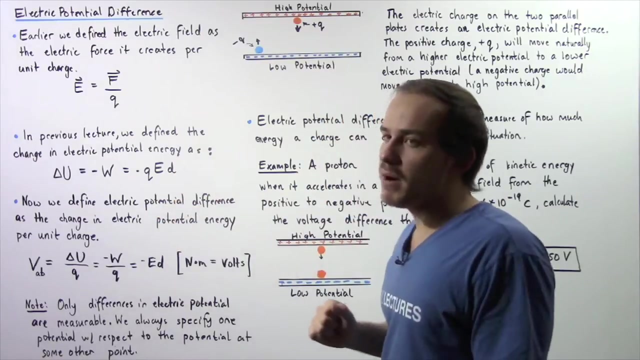 And notice that Q's will cancel top and bottom and we're left with E multiplied by D. So the voltage difference when our electric field is assumed to be constant is equal to the electric field multiplied by the distance between point A and point B. Now the units of voltage are newtons multiplied by meters, and this has a specific name that. 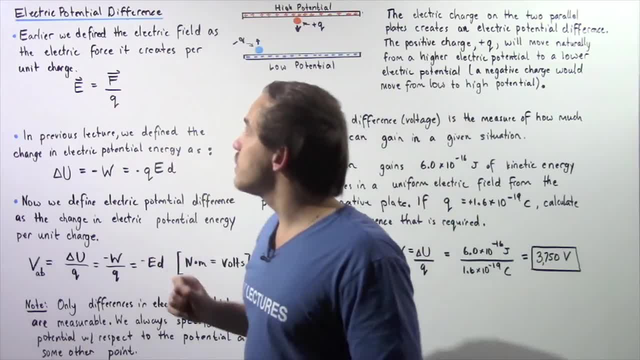 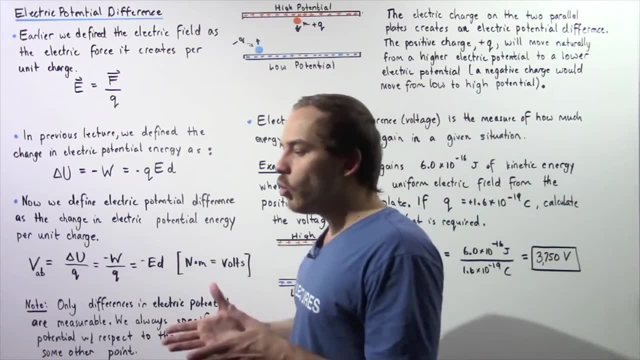 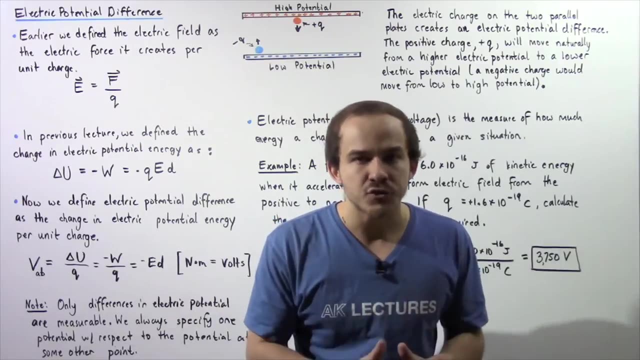 is called volts, And that's exactly why we call the electric potential difference the voltage difference. Now, in the same exact way that only a difference in potential energy is measurable, only a difference in voltage is measurable, and that's why we discuss voltage difference and not simply. 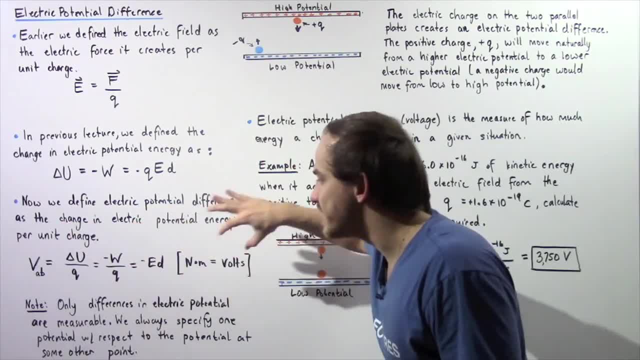 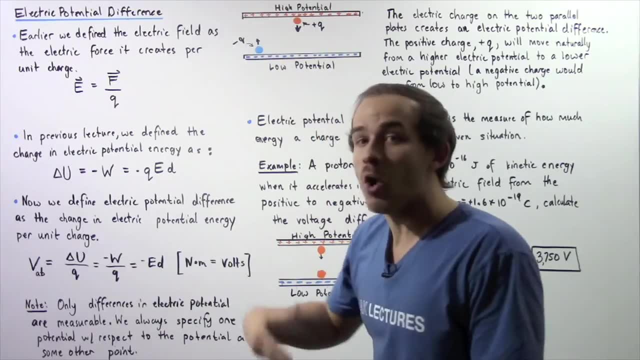 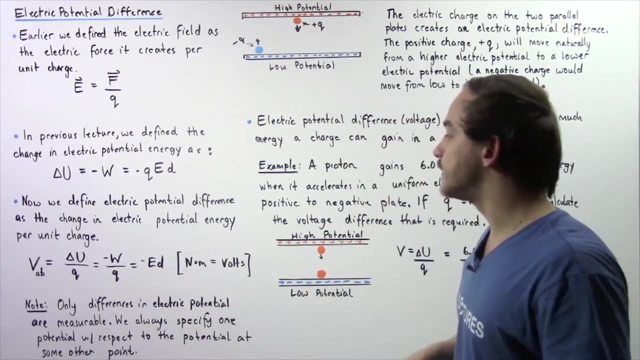 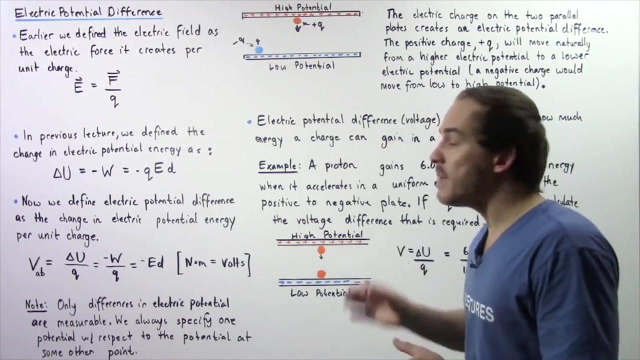 voltage. So only differences in electric potential or voltage are measurable. We always specify one electric potential, one voltage, with respect to another electric potential with another voltage at some other point. So let's suppose we have the following diagram: we have the following setup: We have two parallel plates. 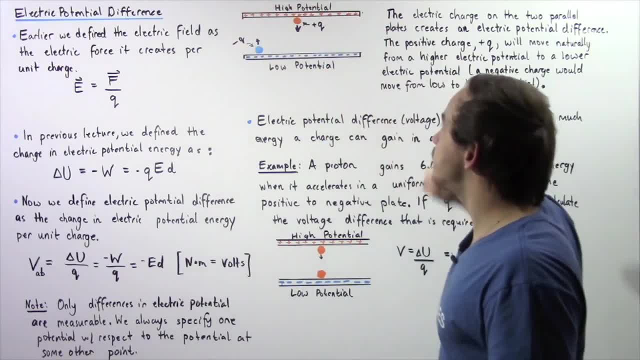 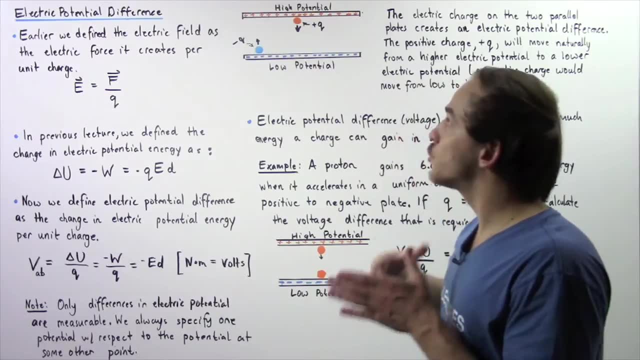 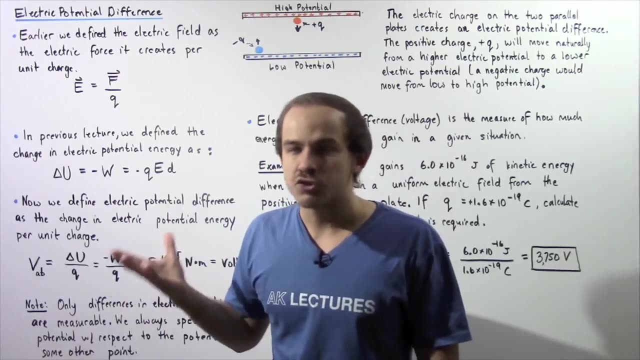 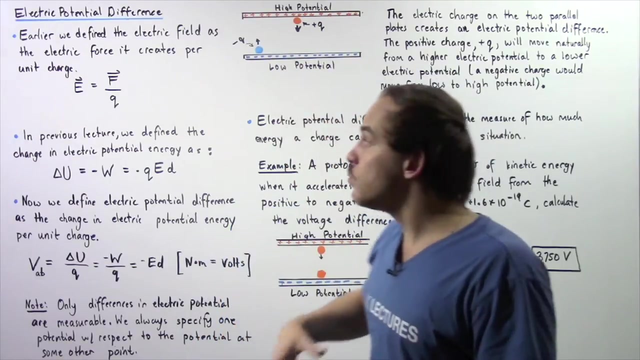 This is our positive parallel plate and this is our negative parallel plate. Now, how exactly is our electric potential difference created? Well, this positive plate is defined to have a high potential, a high electric potential, And this negative plate is defined to have a low electric potential. 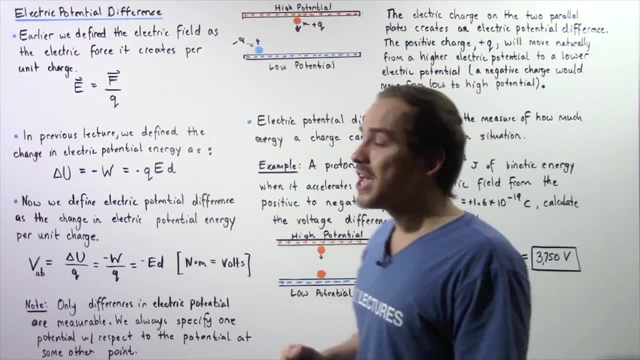 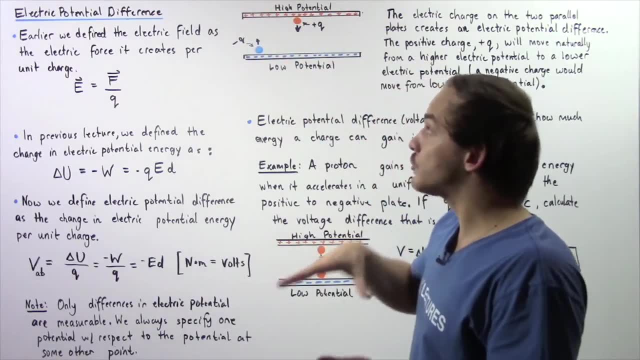 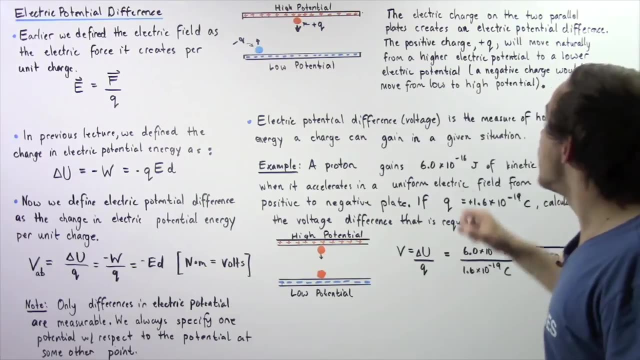 And what actually creates the electric potential difference is the difference in charge. We have a positive charge and we have a negative charge and that creates an electric potential difference because there is a distance separating these two charges. So the electric charge on the two parallel plates creates an electric potential difference. 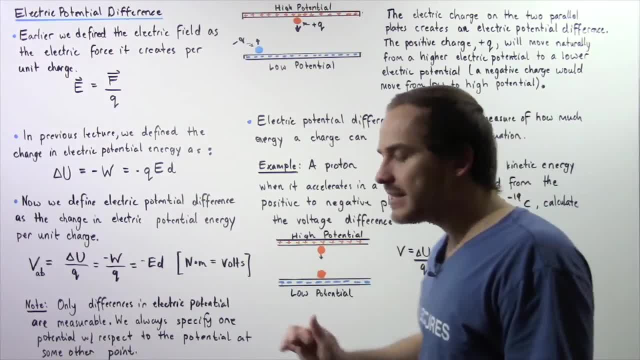 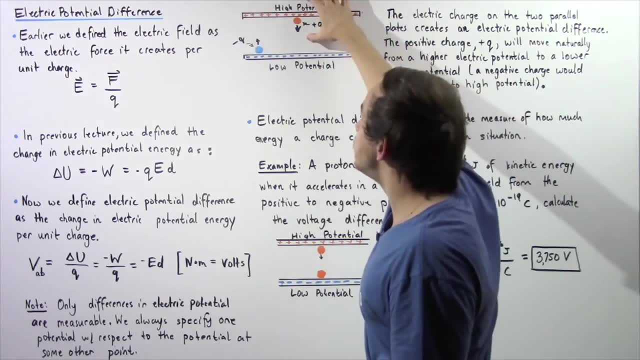 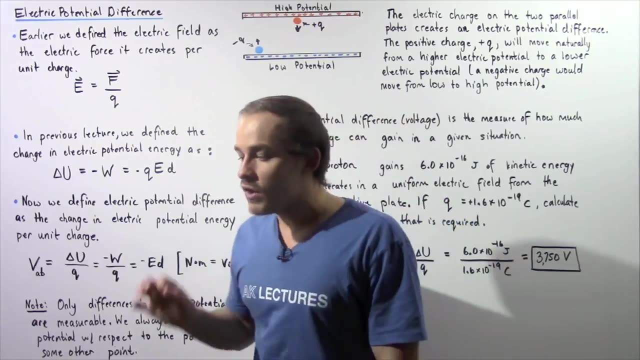 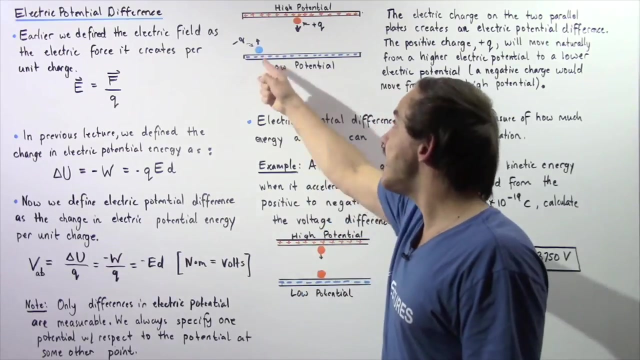 Now, if we take a positive charge and we place it by this positive plate, our charge will move from the high potential to the low potential, and that is always true. A positive charge will always move from a high voltage to a low voltage, but an electron, because it has, or a negative charge, because it has the opposite sign, will move in the 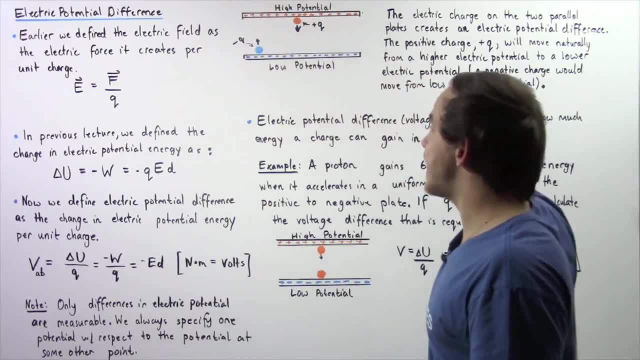 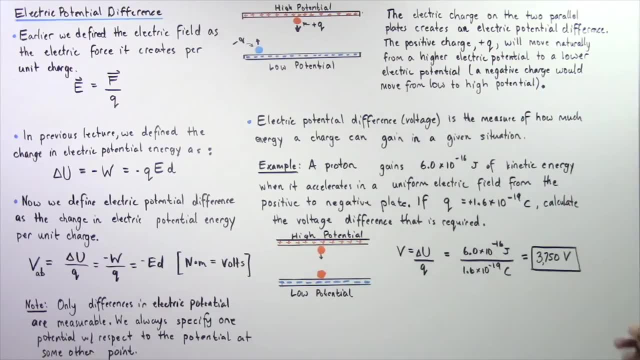 opposite direction. It will always move from the low potential to our high potential. So the positive charge given by positive Q will move naturally from a high electric potential to a lower electric potential. On the other hand, a negative charge given by negative Q will move from the low potential. 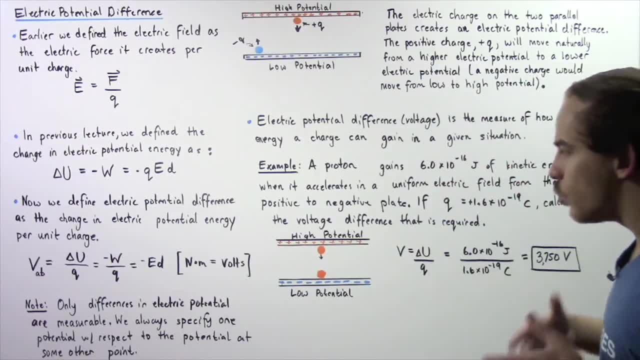 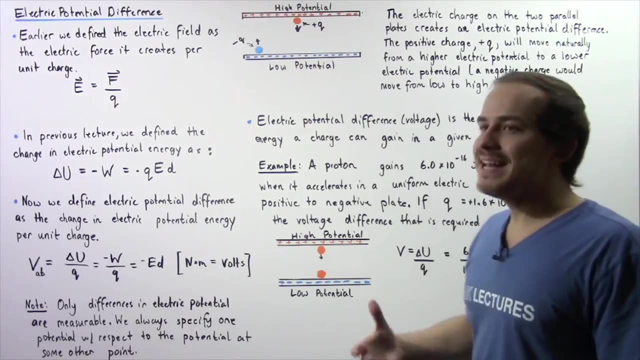 to the high potential. Now another useful way of defining electric potential difference is in the following: Electric potential difference, or the voltage difference, is the measure of how much energy a charge can gain in a certain situation. So let's look at the following: positive electric charge. 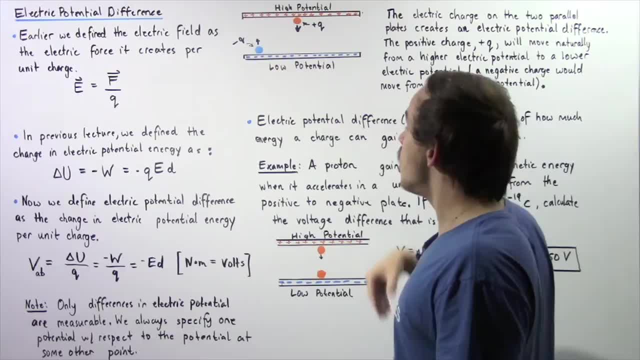 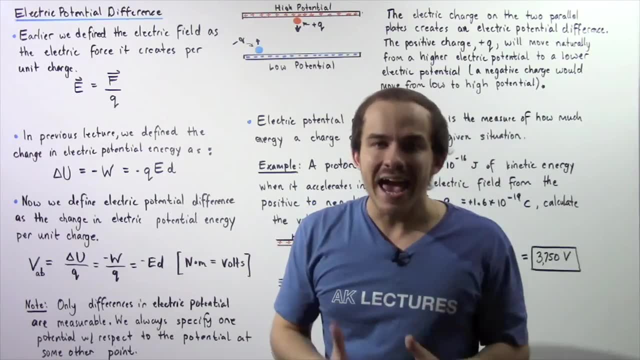 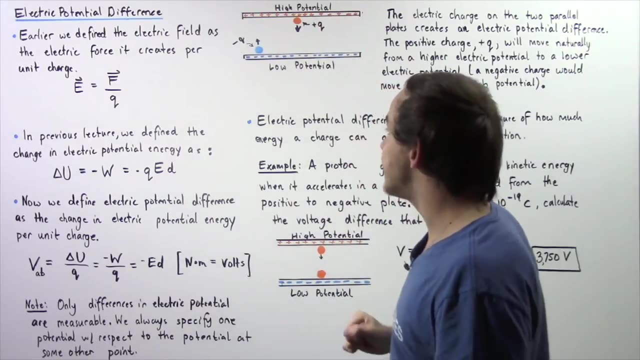 When it travels from the high potential to the low potential. when it travels in this voltage difference, it gains energy. It gains kinetic energy. at the same exact time When this negative charge moves from the low potential to the high potential, because there exists a voltage difference- this charge will gain energy. 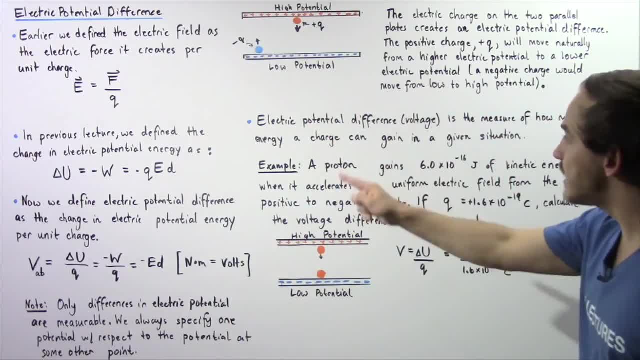 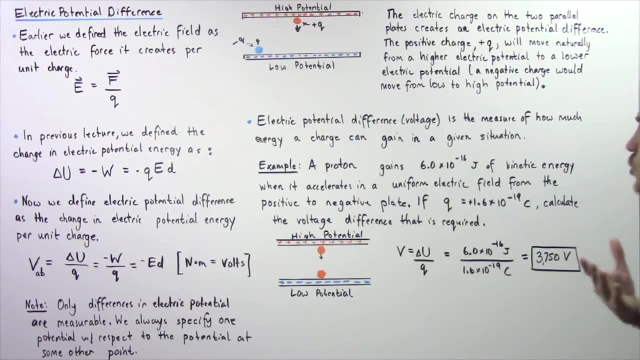 It will gain kinetic energy. So once again, electric potential difference or voltage difference is the measure of how much energy a certain electric charge can gain in a certain field, in a certain electric field. Now let's look at the following example: A proton gains 6.0 times 10 to the negative 16 joules of kinetic energy when it accelerates. 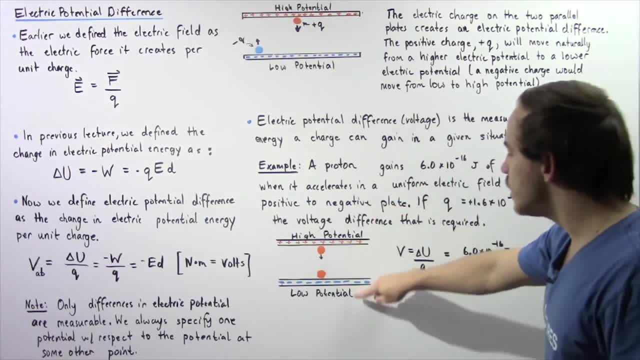 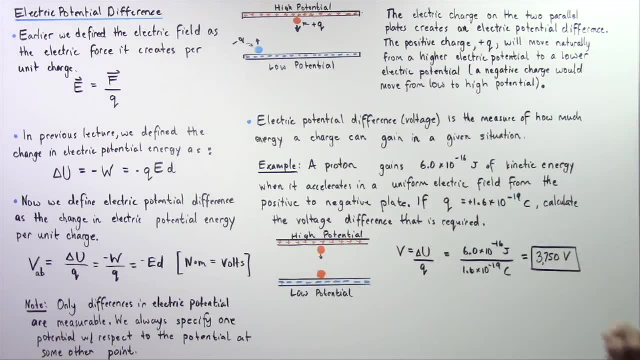 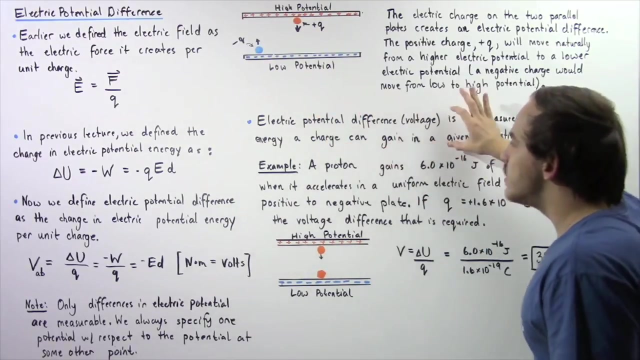 in a uniform electric field from the positive to the negative plate, as shown in the following diagram. If the charge of our proton is positive 1.6 times 10 to the negative, 19 coulombs calculate the voltage difference that is required. Remember: the only way that this proton gains energy is because there must exist an electric 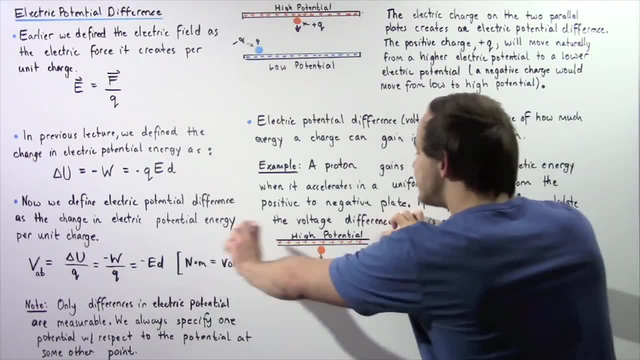 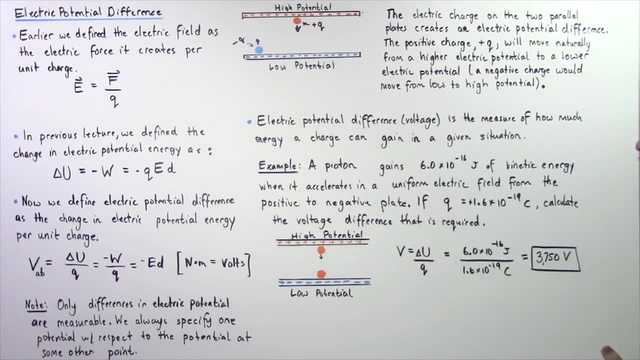 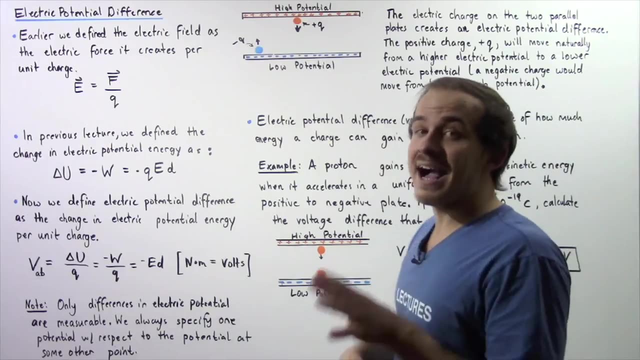 potential difference or a voltage difference between this positive plate and this negative plate. So that's exactly how we defined the electric potential difference. So when our proton moves from the high potential to the low potential, it will gain kinetic energy. So to calculate how much electric potential it gains: 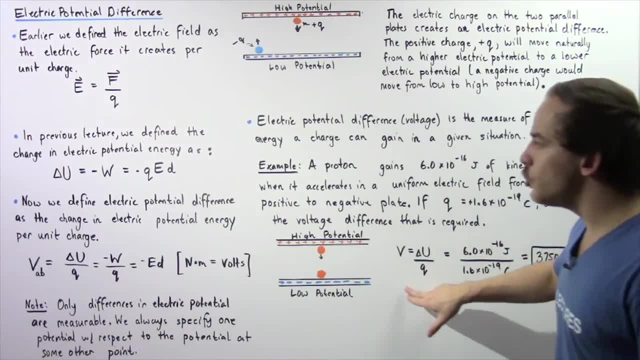 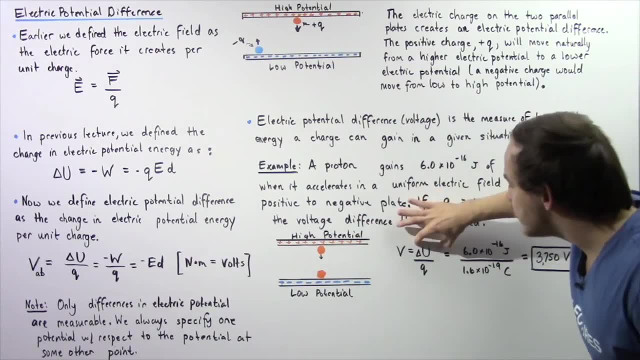 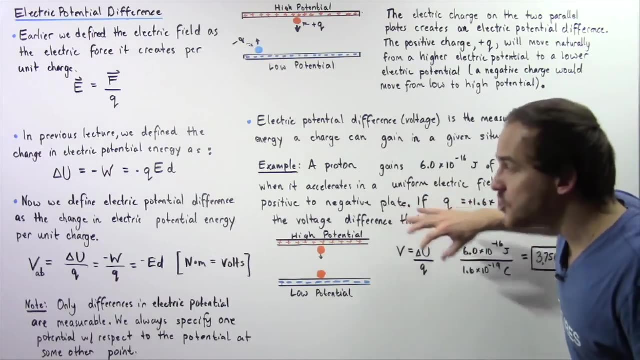 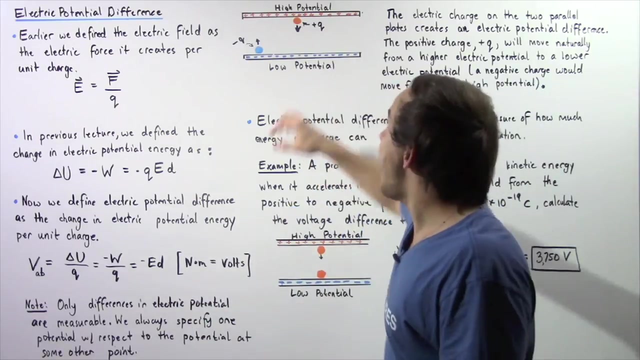 How much electric potential difference we must have. we use this equation, So our voltage difference is equal to how much energy it has to gain, divided by Q. Now, actually, this is how much potential energy it has to lose because the electric potential energy is transformed into kinetic energy as this charge moves from the high potential. 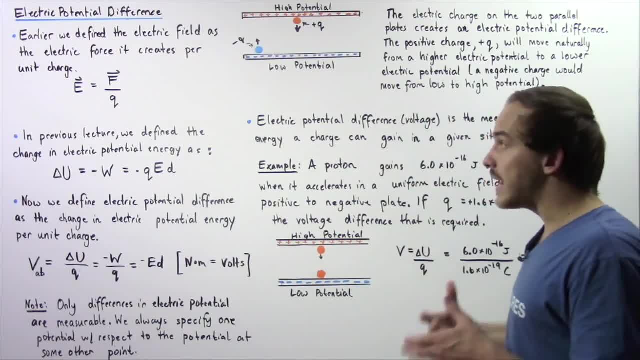 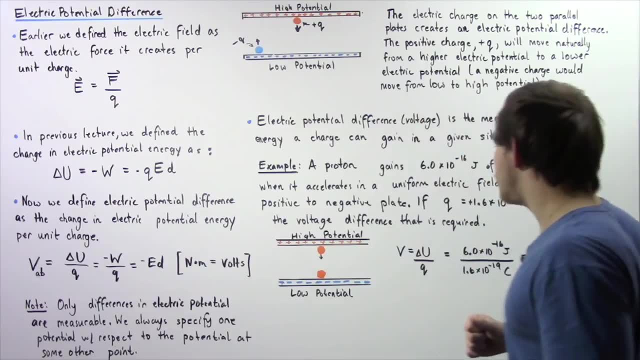 to the low potential. So the amount of electric potential energy that our charge, our proton, loses is equal to the amount it gains in kinetic energy. So our change in U is simply 6.0 times 10 to the negative 16 joules. 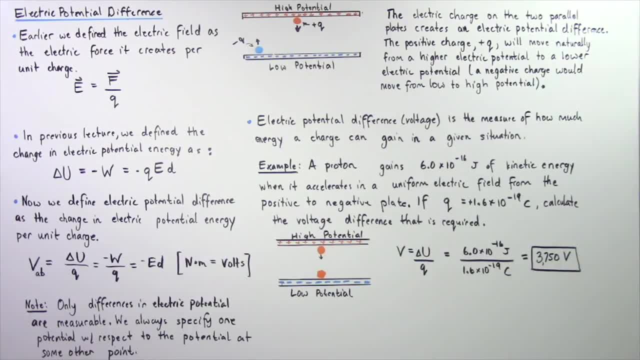 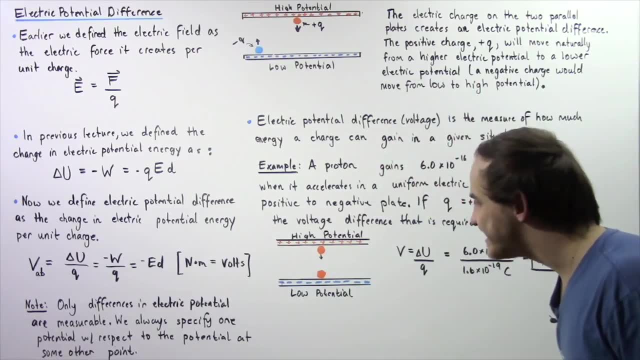 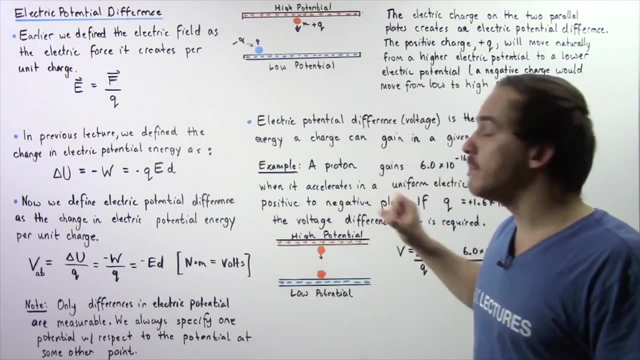 We divide by the charge, and that gives us 3,750 volts. is our voltage difference or the electric potential difference that must exist for this proton to gain this quantity of energy. So that's exactly how we define the electric potential difference. So we can calculate the electric potential difference as we move from the high potential. to the low potential. 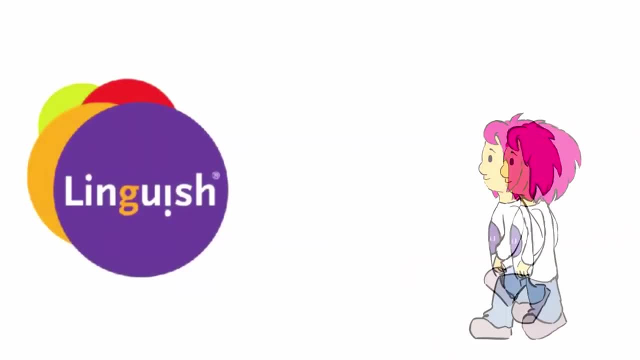 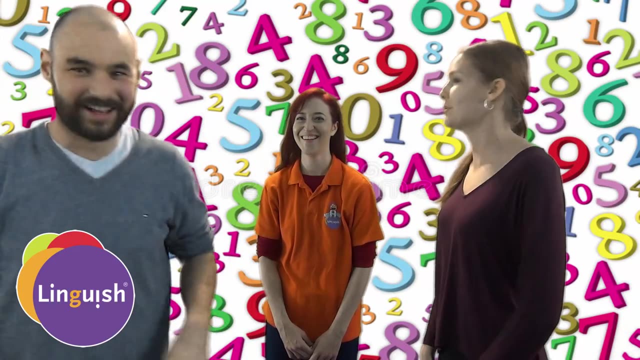 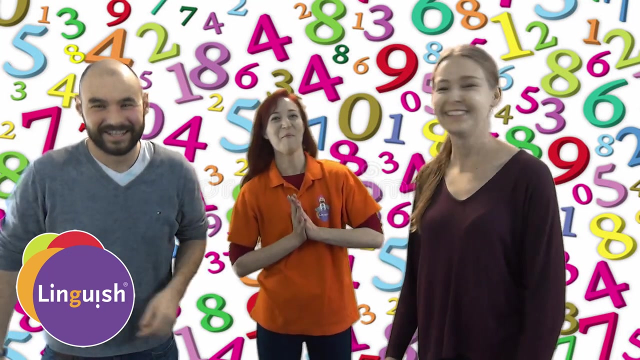 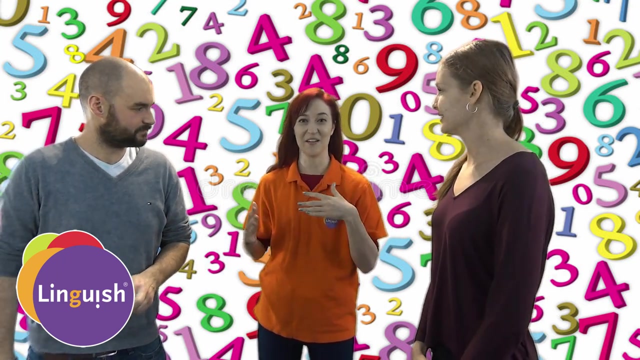 3,, 17,, 20 are all the numbers you could use in the counting game. But if you're using, if it's for little kids, I would say keep it from 1 to 10.. If it's older kids, you can. 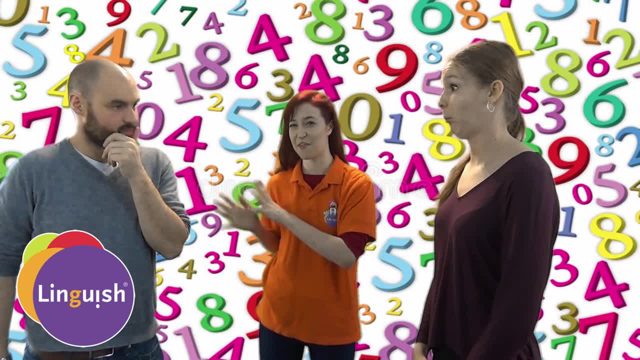 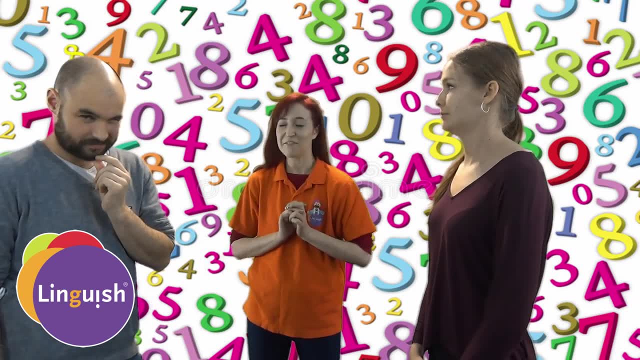 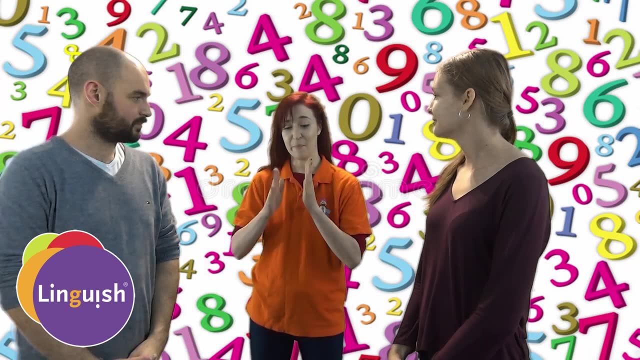 not do numbers. You could do ordinals like first, second, third make it more difficult. So counting game is really easy, but they will find it difficult. All you have to do is count from 1 to 10. But you cannot say the numbers after each other from the same. 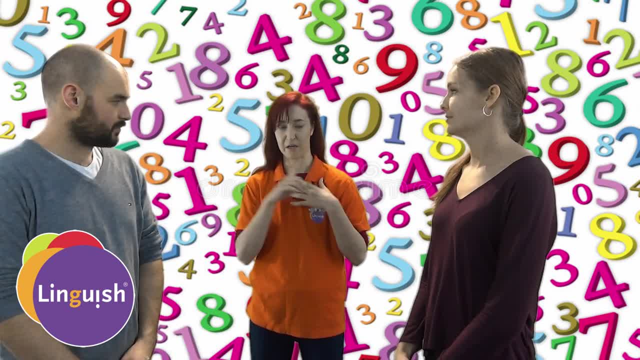 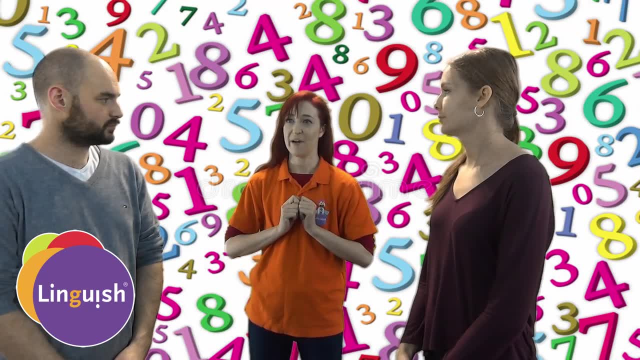 person. So if I was to start, I can't say 1,, 2,, because that's two numbers. I can only say one number, And if you say the same number at the same time, we have to go all the way.